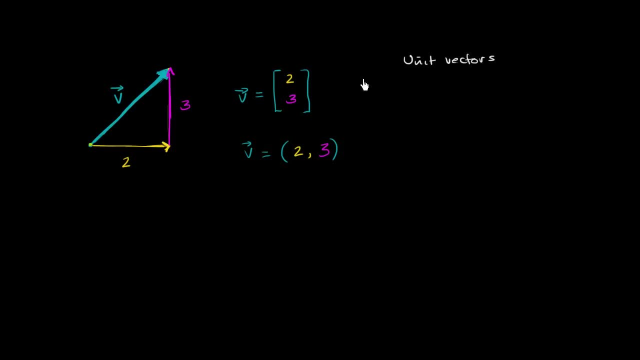 And the way that we denote that it is a unit vector is, instead of putting an arrow on top, we put this kind of hat on top of it. So the unit vector i. if we wanted to write it in this notation right over here. 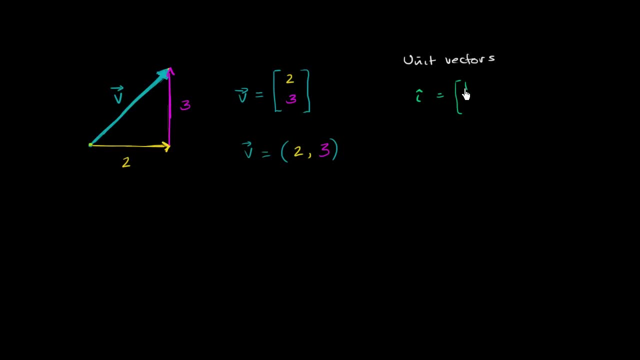 we would say: it only goes one unit in the horizontal direction and it doesn't go at all in the vertical direction. So it would look something like this: It would look something like that: So that's the unit vector i, And then we can define another unit vector. 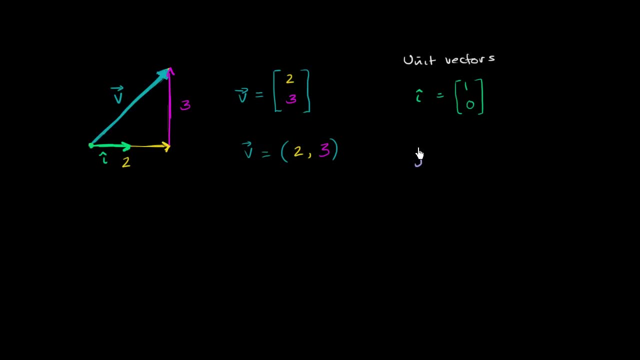 Let's call that unit vector, or it's typically called j, which would go only in the vertical direction and not in the horizontal direction, And it goes one unit in the vertical direction. So this went one unit in the horizontal. Now j is going to go one unit in the vertical. 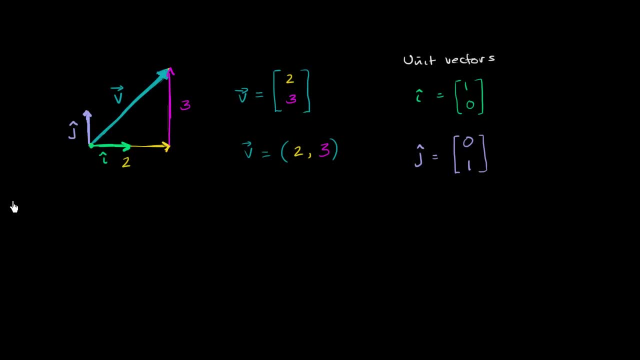 So j just like that. Now, Any vector, any two-dimensional vector, we can now represent as a sum of scaled-up versions of i and j. And you say: well, how do we do that? Well, you could imagine vector v, right here. 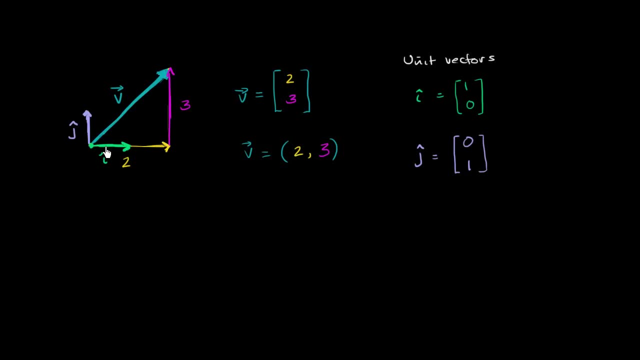 is the sum of a vector that moves purely in the horizontal direction that has length 2, and a vector that moves purely in the vertical direction, that has length 3.. So we could say that vector v. Let me do it in that same blue color. 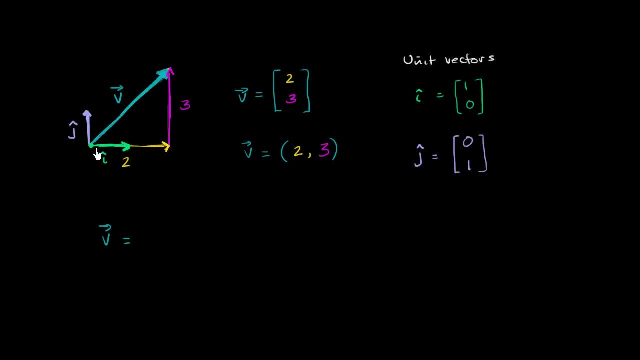 Vector v is equal to. So if we want a vector that has length 2 and it moves purely in the horizontal direction, well, we could just scale up the unit vector i. We could just multiply 2 times i. So let's do that. 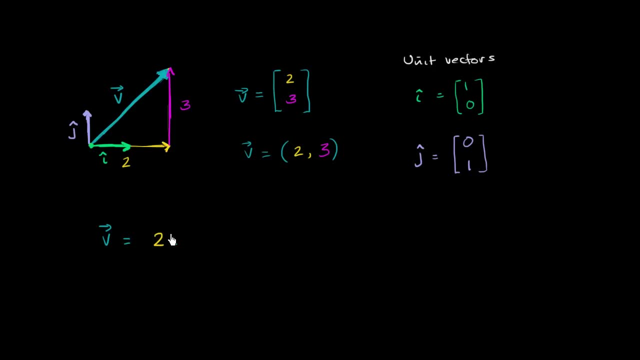 It's equal to 2 times our unit vector i. So 2i is going to be this whole thing right over here Or this whole vector. Let me do it in this yellow color. This vector right over here You could view as 2i. 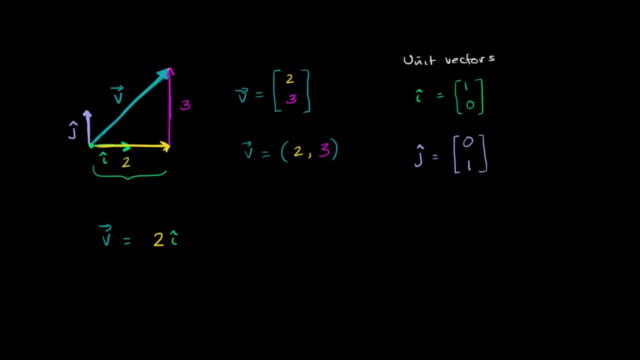 And then to that we're going to add 3 times j. So plus 3 times j. Let me write it like this: Let me get the color: 3 times j, Once again 3 times j. is going to be this vector right over. 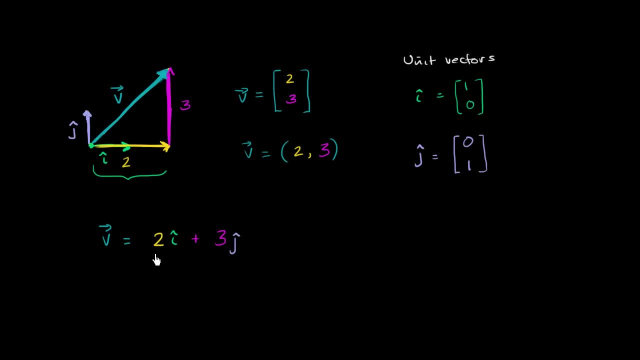 here. And if you add this yellow vector right over here to the magenta vector Notice, we're putting the tail of the magenta vector at the head of the yellow vector. And if you start at the tail of the yellow vector and you go all the way to the head of the magenta vector, 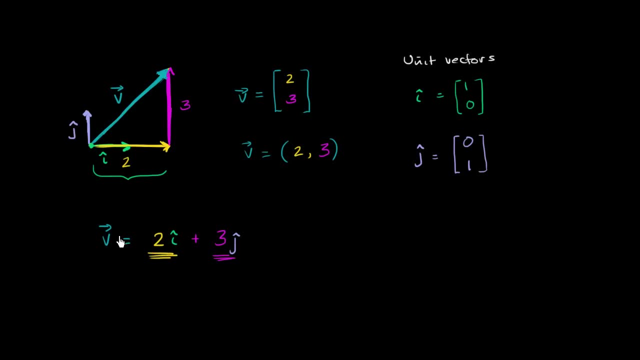 you have now constructed vector v. So vector v, you could represent it as a column vector like this: 2, 3.. You could represent it as 2 comma 3.. Or you could represent it as 2 times i, with this little hat over it, plus 3 times j. 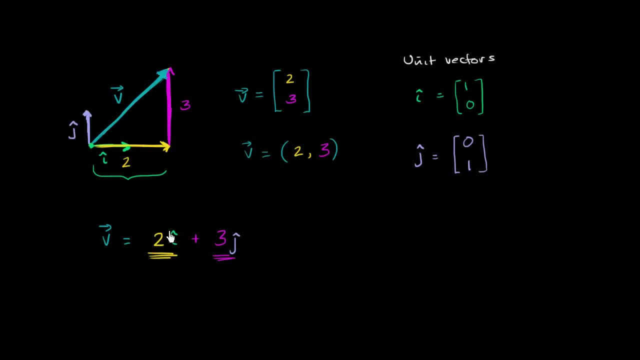 with this little hat over it, i is the unit vector in the horizontal direction. Let's do that, Let's do that. So i is the unit vector in the positive horizontal direction. If you want to go the other way, you would multiply it by a negative. 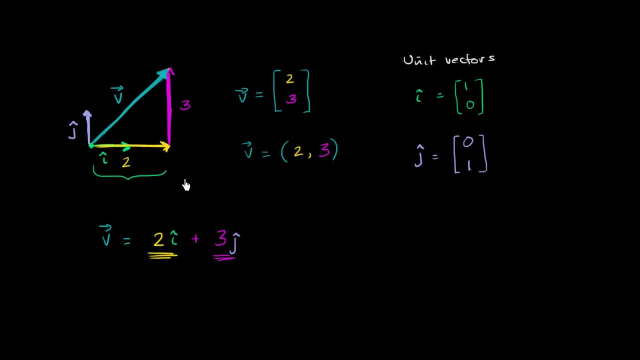 And j is the unit vector in the vertical direction, As we'll see in future videos, once you go to three dimensions you'll introduce a k, But it's very natural to translate between these two things. Notice 2, 3,, 2, 3.. 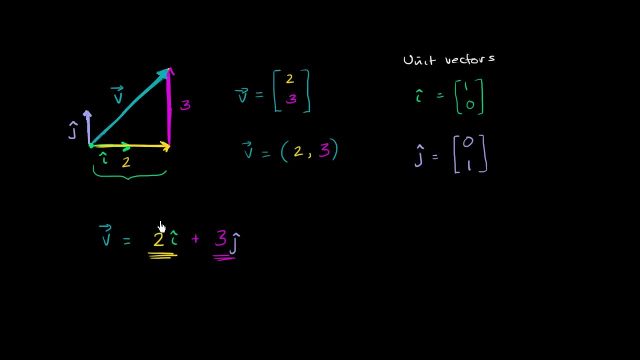 And so with that, let's actually do some vector operations using this notation. So let's say that I define another vector. Let's say it's vector b And vector b is equal to. I'll just come up with some numbers here: vector b is equal to negative 1 times i. 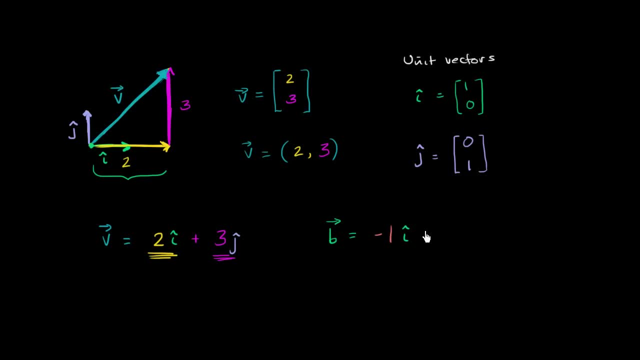 times the unit vector i plus 4 times the unit vector in the horizontal direction. So, given these two vector definitions, what would the vector, what would be the vector v plus b be equal to? I encourage you to pause the video and think about it. 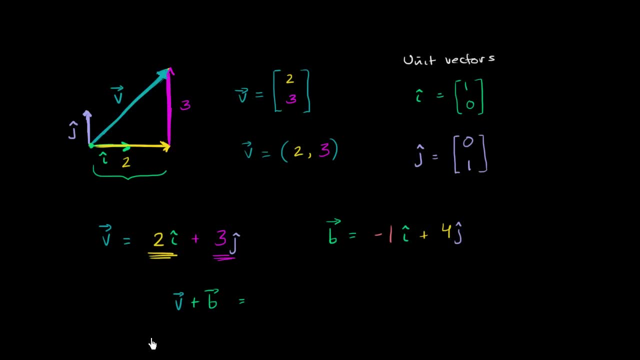 Well, once again, we just literally have to add corresponding components. We could say: OK, well, let's think about what we're doing in the horizontal direction. We're going 2 in the horizontal direction here, And now we're going negative 1.. 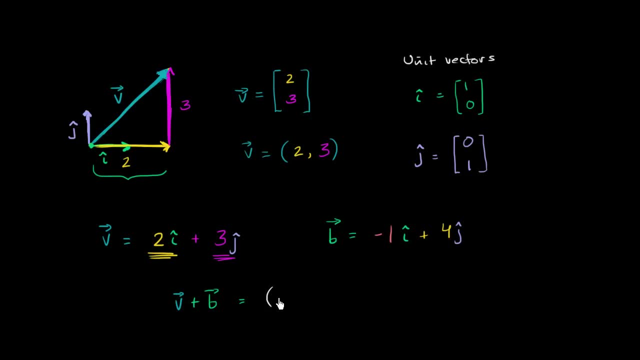 So our horizontal component is going to be 2, 2 plus negative 1 in the horizontal direction And we're going to multiply that times the unit vector i. And this once again just goes back to adding the corresponding components of the vector. 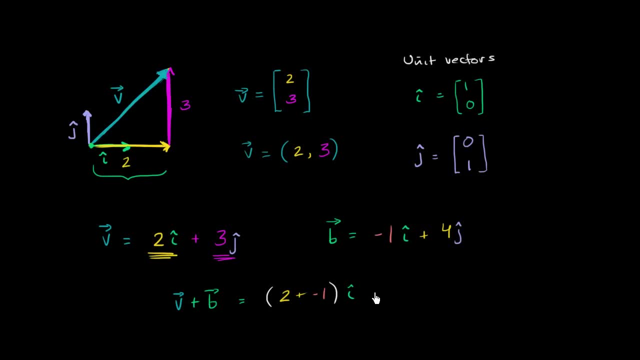 And then we're going to have plus 4, plus 4, or plus 3 plus 4.. Let me write it that way: Plus 3 plus 4 times the unit vector j in the vertical direction, And so that's going to give us 2.. 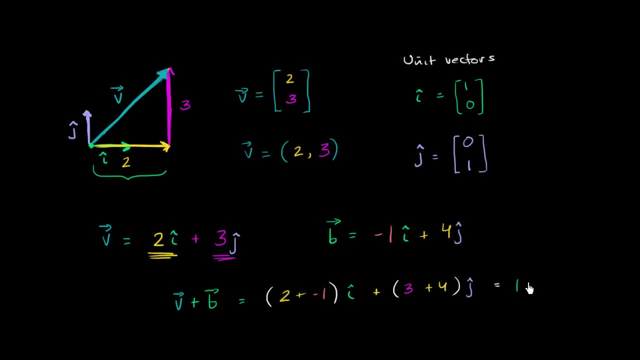 I'll do this all in this one color: 2 plus negative 1.. 1 is 1.. i And we could literally write that just as i. Actually, let's do that, Let's just write that as i. But we got that from: 2 plus negative, 1 is 1.. 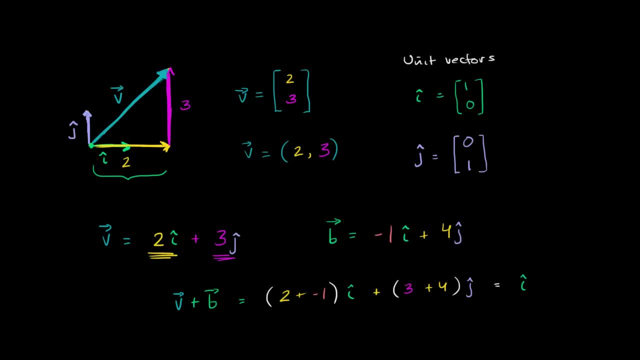 1 times the vector is just going to be that vector Plus 3 plus 4 is 7. 7j And you see, this is exactly how we saw vector addition in the past is that we could also represent vector b like this: 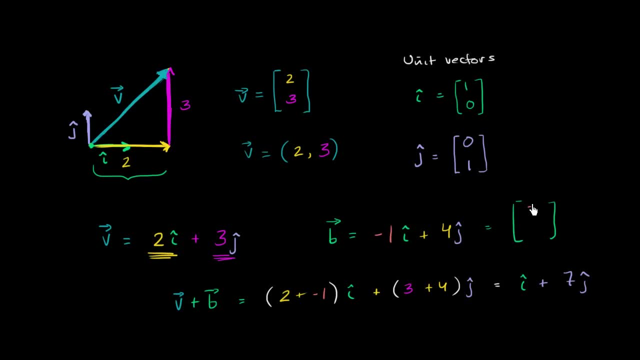 We could represent it like this: Negative 1.. Negative 1, 4.. Negative 1, 4.. And so if you were to add v to b, you add the corresponding terms. So this should be equal to: if we 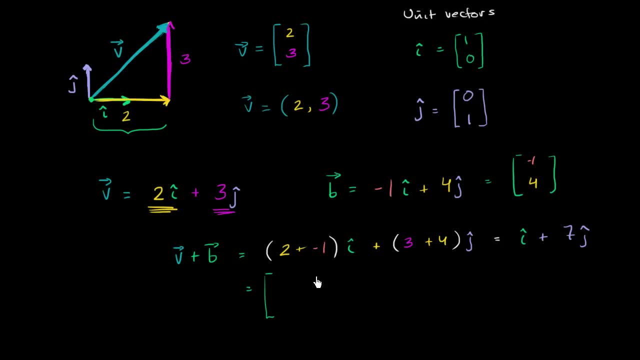 were to add corresponding terms. looking at them as column vectors, that is going to be equal to 2 plus negative 1, which is 1.. 3 plus 4 is 7.. So this is the exact same representation as this. 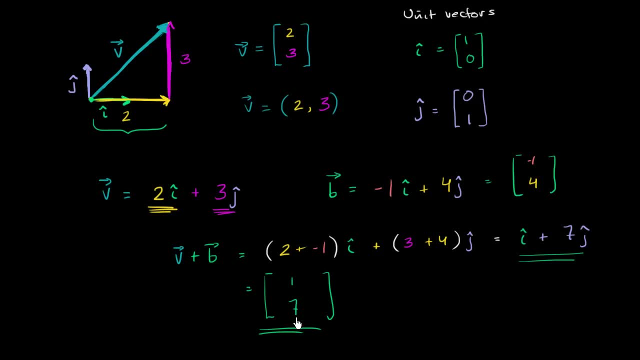 This is using unit vector notation And this is representing it as a column Column vector. 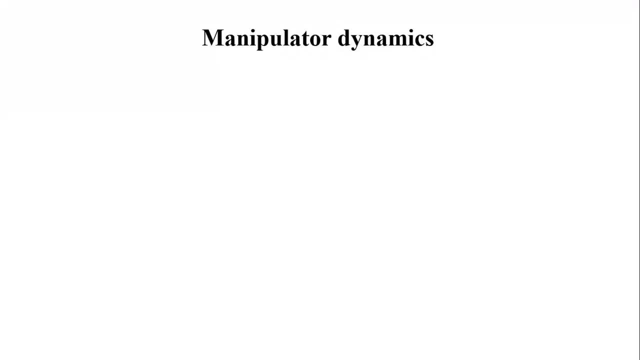 Hi, let's discuss manipulator dynamics. Manipulator dynamics deals with the relationship between forces acting on robot and the accelerations they produce. Manipulator dynamics is written in this form, similar to this, in this form, and you can see that the right hand side of this relation.